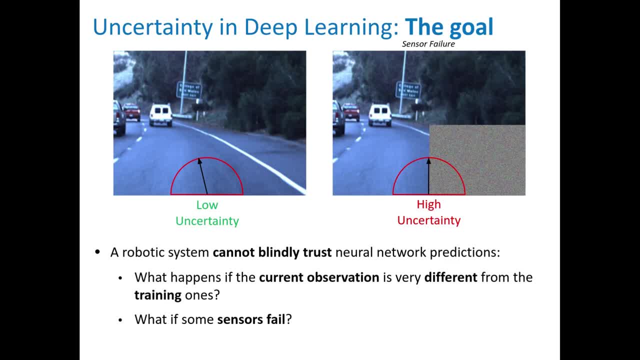 However, a robot cannot blindly trust the prediction of a neural network. In fact, what happens if the current observation is very different from the training ones? Or what if some of these sensors fail A wrong prediction because of this can be very problematic for a robot and also for the surrounding of it. 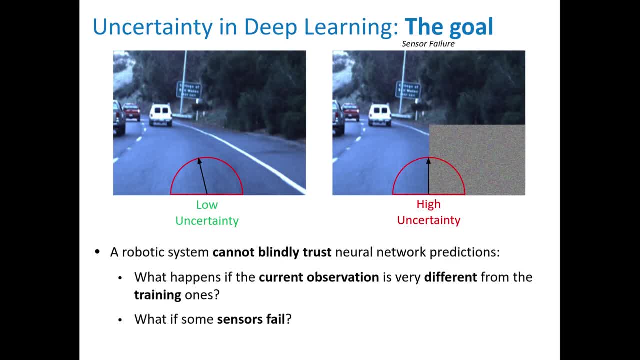 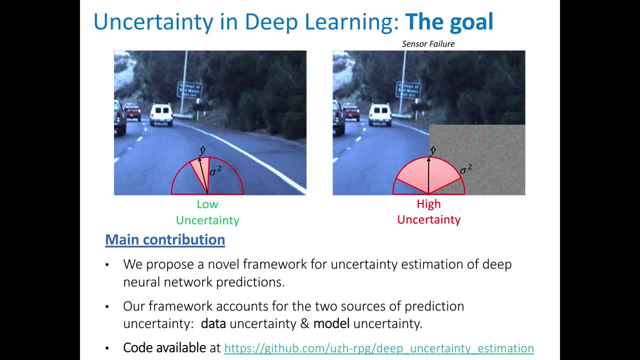 Think, for example, about an autonomous car. To detect and avoid this wrong prediction, we propose a general framework for uncertainty estimation of deep neural networks. In deep neural networks, our framework can model the uncertainty in neural networks coming from two sources: Data uncertainty and model uncertainty. 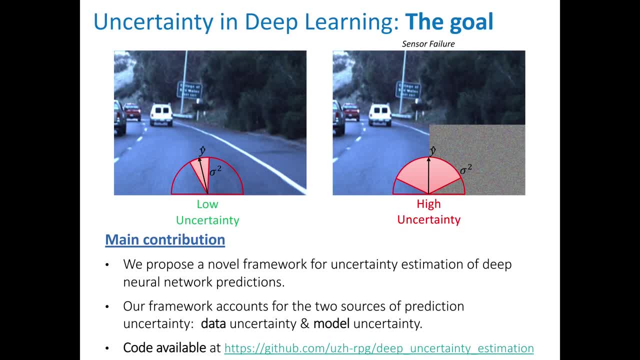 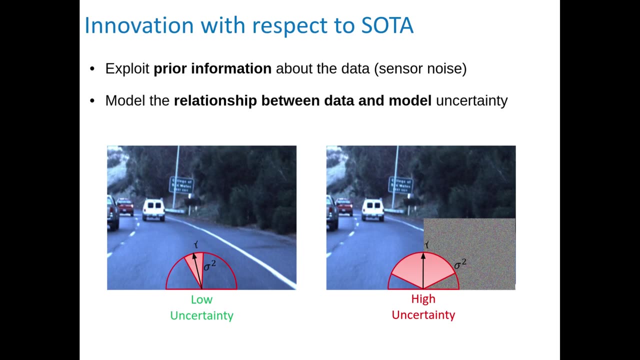 The data uncertainty should be a model of uncertainty. The data uncertainty should be a model of uncertainty. The data uncertainty usually describes the uncertainty coming from the sensor noise, while the model uncertainty describes how much a neural network is uncertain about its own prediction. With respect to state-of-the-art, we propose two major innovations. 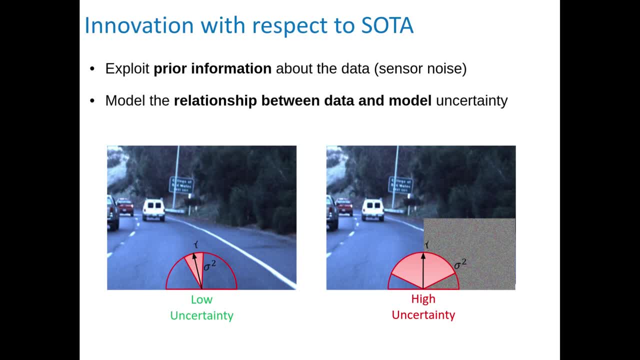 First, we propose to use prior information about the data that a robot has in the form of sensor noise to predict better uncertainty. Second, we propose to use prior information about the data that a robot has in the form of sensor noise to predict better uncertainty. 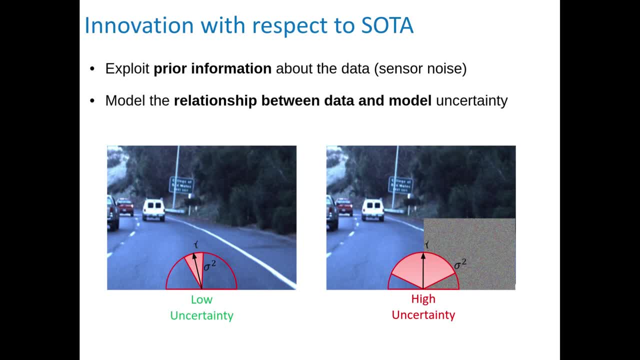 Third, we propose to use prior information about the data that a robot has in the form of sensor noise to predict better uncertainty. And also we propose to model the relationship between the two uncertainties- the data and the model- to better predict the total uncertainty of a neural network. 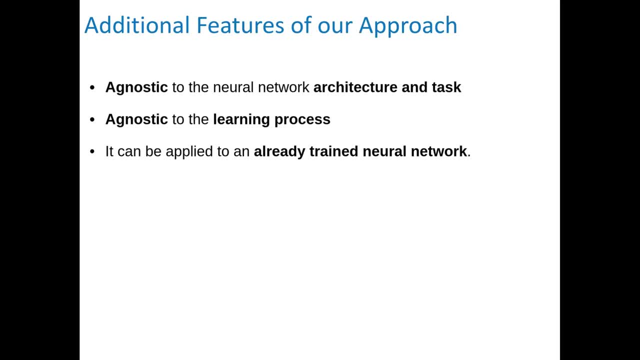 In addition, our framework has some interesting features. In particular, it is agnostic to the neural architecture and task. It is also agnostic to the learning process. That means it can be applied to any training procedure and also it can be applied to already trained neural networks. 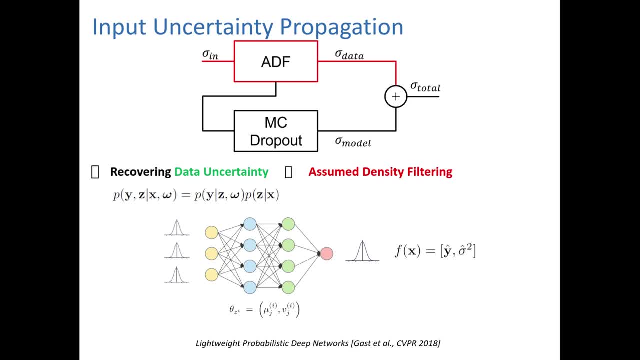 To model the data uncertainty we use assumed density filtering. Specifically, we fit every neural network node with a Gaussian distribution and set the input value of the neural network node and set the input value of the neural network node. And set the input value of the neural network node. 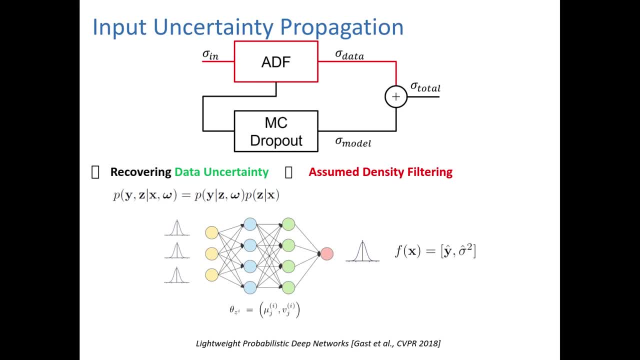 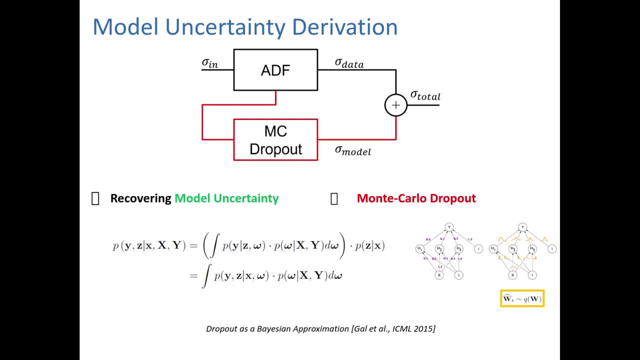 With the noise coming from the sensor cheat sheet. With the noise coming from the sensor cheat sheet. In addition, we compute model uncertainty using Monte Carlo Dropout, Which basically boils down to create Bayesian belief networks, which basically boils down to create Bayesian belief networks. uncertainty, putting a probability distribution on every of the network weights. 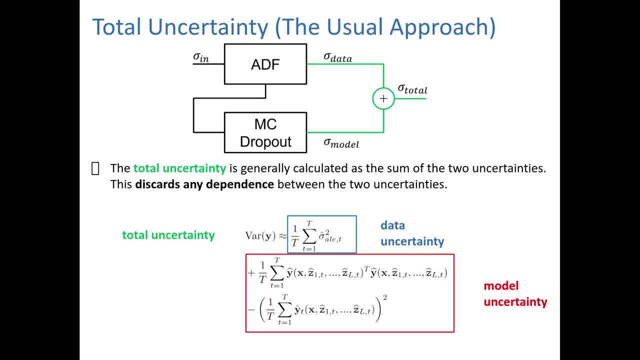 The usual approach for finding the total uncertainty is just to sum the two. So data uncertainty, model uncertainty, just sum them. However, this approach, which is usually done, discards any dependencies between the data and model uncertainty. But this is fundamentally wrong, because high sensor noise can also result in high model. 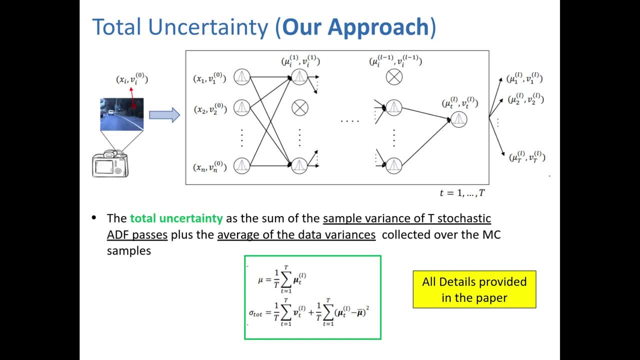 uncertainty. For this reason we propose to compute the total uncertainty as an average of Bayesian networks, Bayesian belief networks, which can account for a better, which can give a better estimate of the total uncertainty with respect to the classical data. So we show a more practical summing approach. 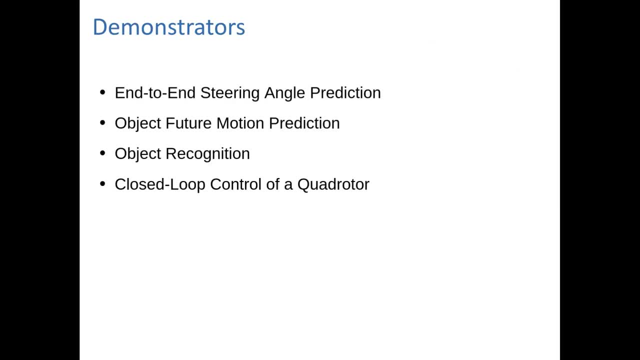 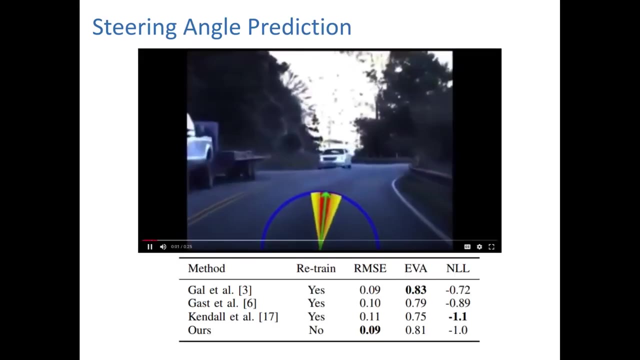 All the details of this are provided in the paper. We demonstrate our framework on four tasks: end-to-end steering angle prediction- object. future motion prediction, object recognition and close-loop control of a quadruple. On steering angle prediction, we adapt an error network used to predict steering angle. 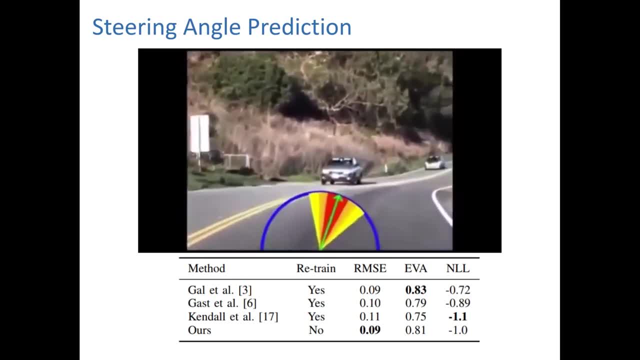 from images and add also uncertainty estimation, The. do you see? Here we have the total uncertainty. The data uncertainty is the number of data that is used. We have a four-point prediction. We have an answer to this. The data uncertainty is the number of data that is used. 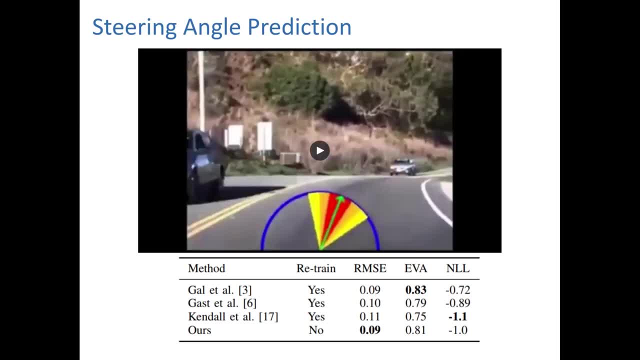 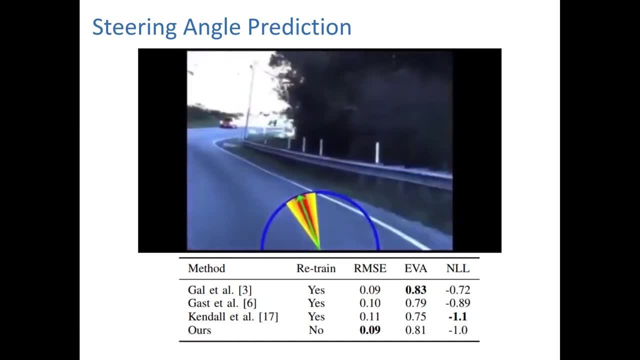 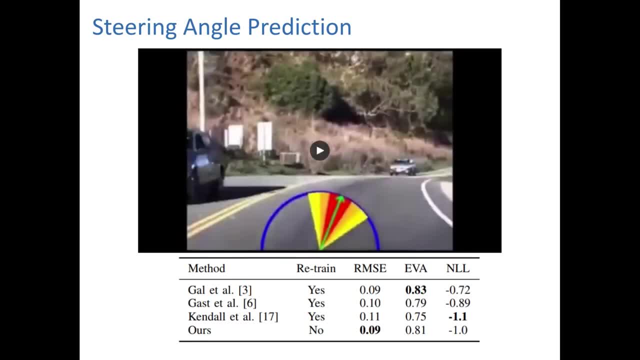 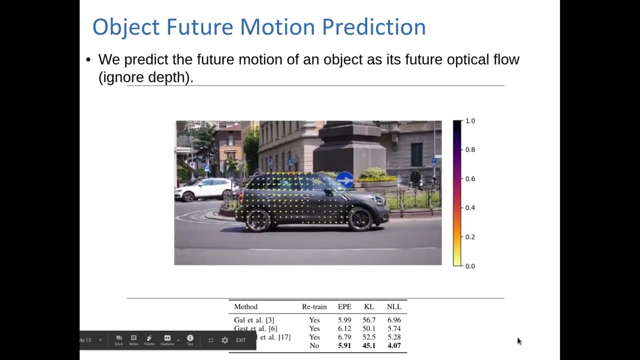 in steering angle, but also very accurate uncertainty estimation, which none of the State-of-the-art methods have at the same time In object-future motion prediction. instead, we predict how an object will move in the future, But of course this also has uncertainty. 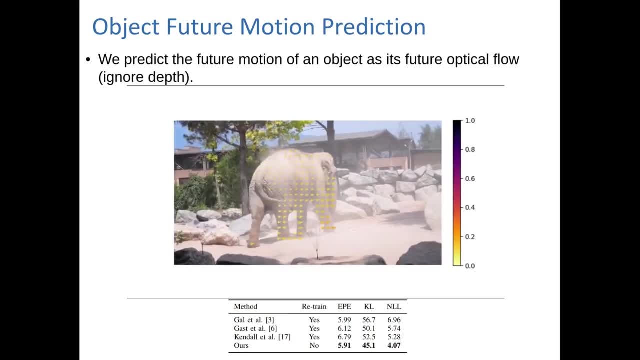 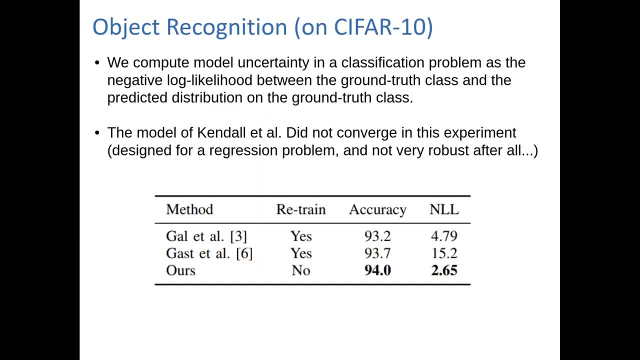 And again we performed this task with higher accuracy and with better uncertainty estimation than State-of-the-art approaches. We also evaluate on an object recognition task on the popular CFAR10 dataset where we again obtain, with respect to previous tasks, with respect to previous 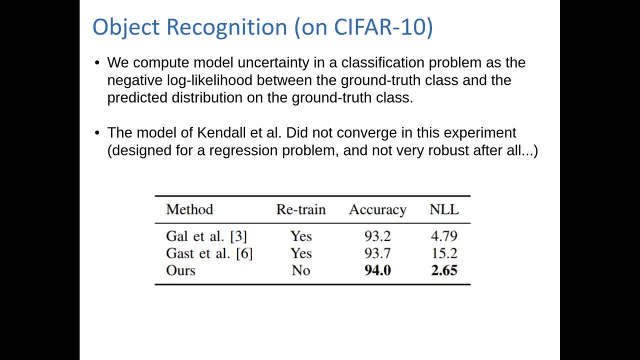 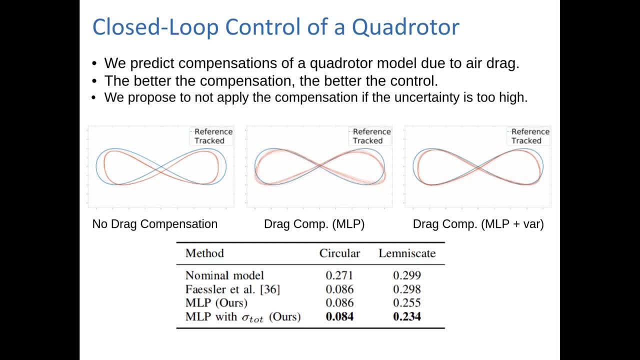 work, a high accuracy estimation and a very good uncertainty fitting. We also studied the problem of closed-loop control of a quadrotor, where we basically showed that keeping uncertainty into consideration for control- specifically, do not apply an action if the neural network is not really sure about it- improves tracking performance. 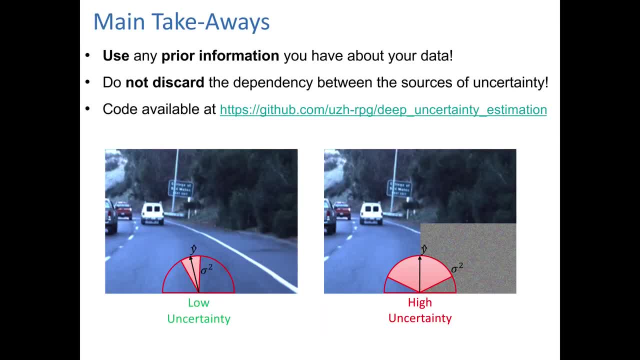 and decreases the odds of a crash. So the main takeaways of our work is that it's important to use any prior information we have about our data and uncertainty estimation, and that's very important for a robotic system, And also it's also fundamental to keep into account. 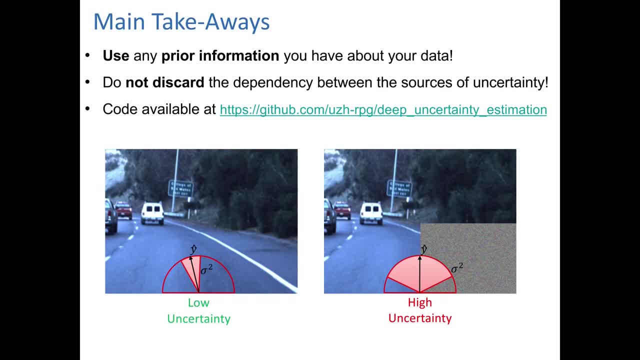 the relationship between the two sources of uncertainty: data and model. Thank you for your attention.